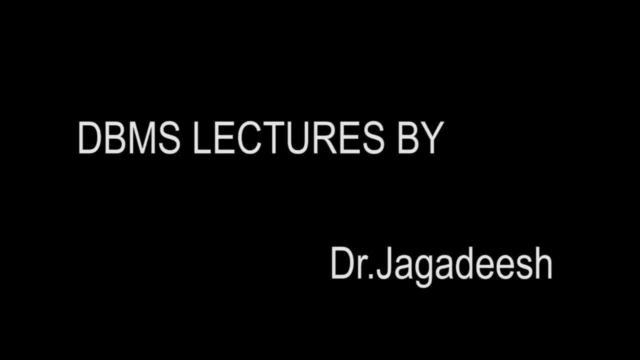 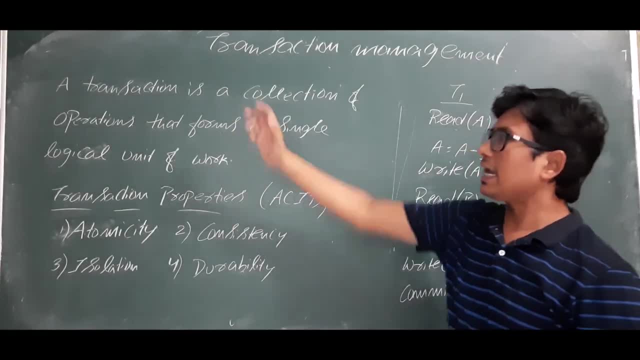 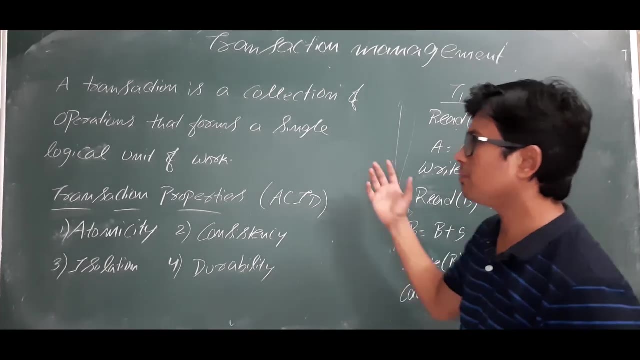 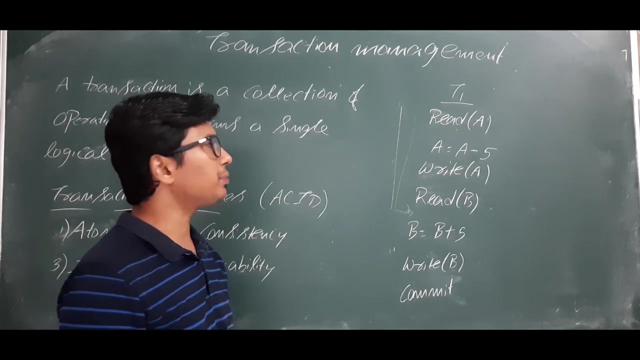 Good morning students. Today we will discuss about transaction management. A transaction is a collection of operations that form a single logical unit of work. Let me give an example for what is a transaction. A transaction here? if you see that we have seven operations, Let me. 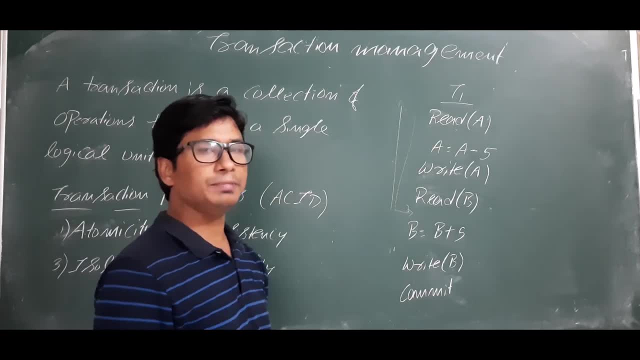 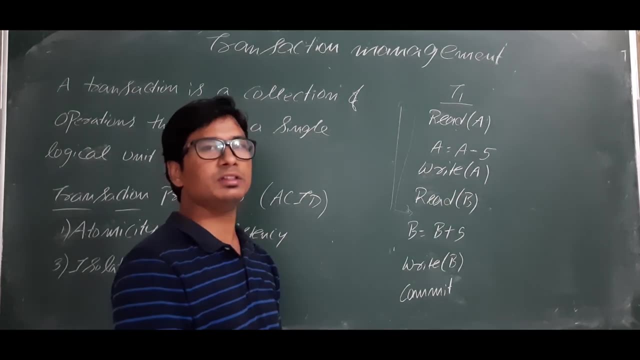 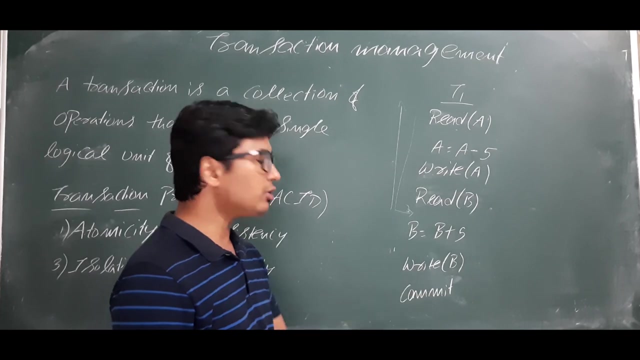 discuss. what is this operation? read a. Read a means we are reading the content from the data item a. Write a is we are temporarily saving the modifications in the memory. Commit operation or we will have abort operation. Commit operation says that you are permanently saving the modifications. 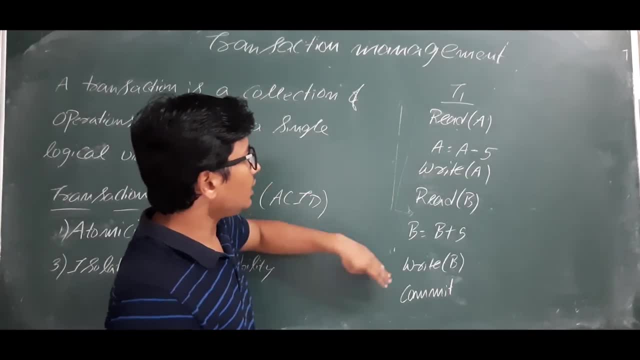 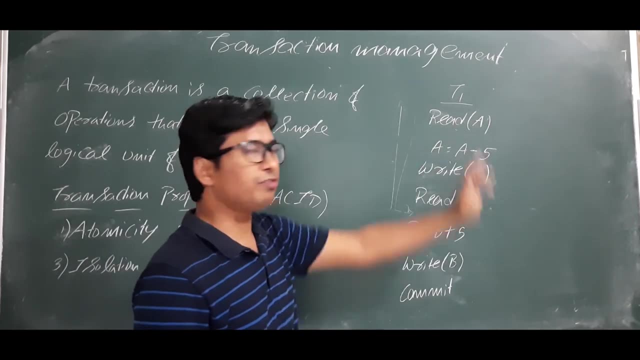 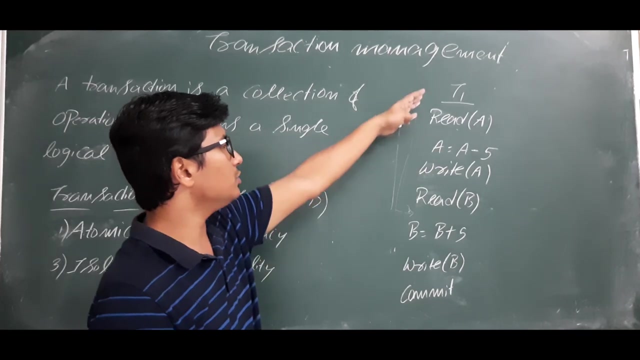 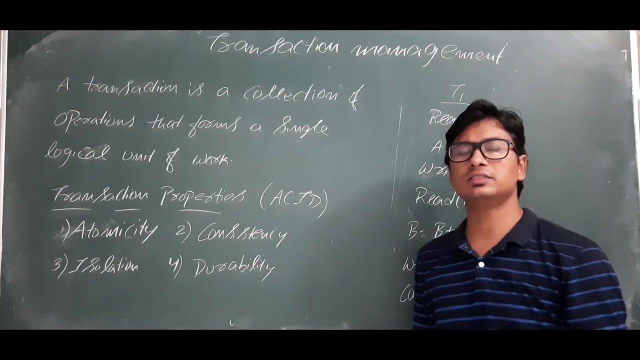 in the database. Now here, what is the operation we are performing is we are subtracting the 5 from a and performing addition 5 to the b. This is the task we are performing using these seven operations. So this one I can call it as a task. Now, each transaction. 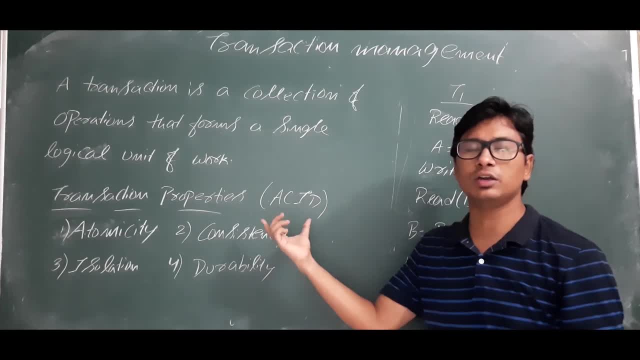 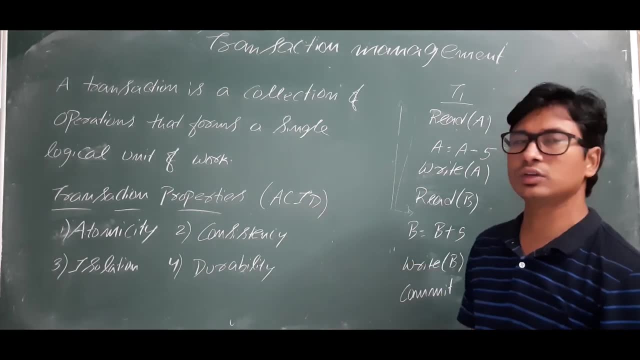 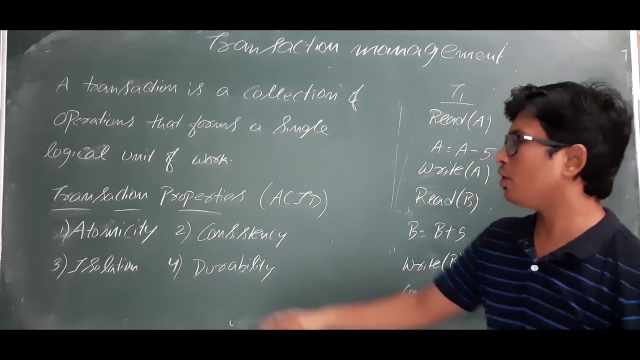 should follow some properties. Those properties we will call it as ACID properties, where a stands for atomicity, c for consistency, i for isolation and d for durability. Let me discuss each property in detail for better understanding. Now, what is atomicity is? if you 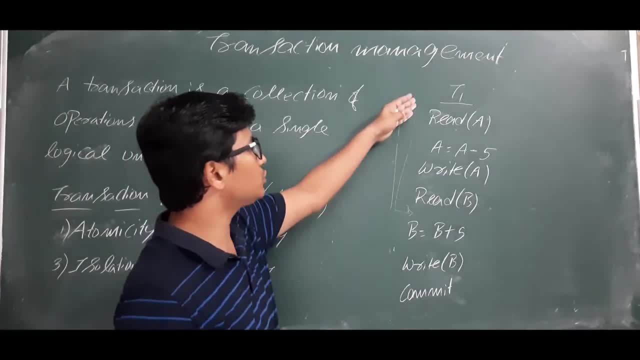 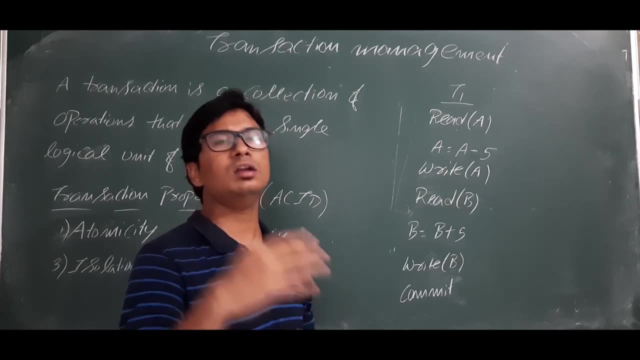 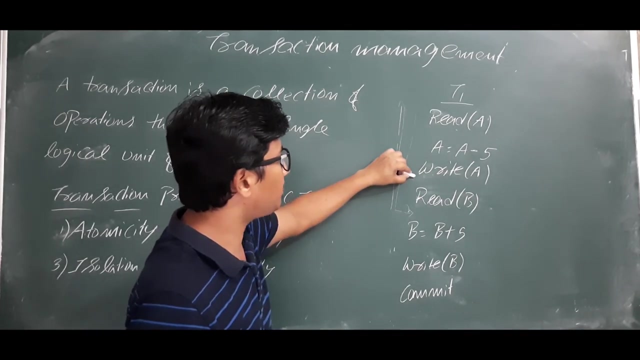 have some seven operations in a transaction, either you should execute all the operation or you should not execute any one. We can simply say that all or none. Suppose let's say that you started executing the transaction. You executed up to three operations Because of some problem, you could 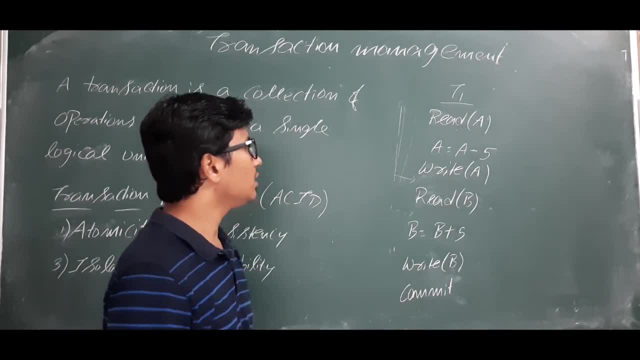 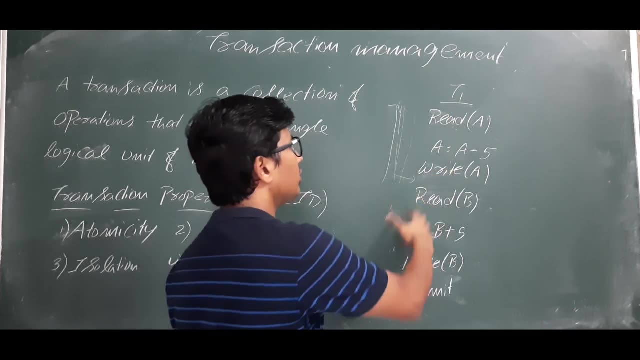 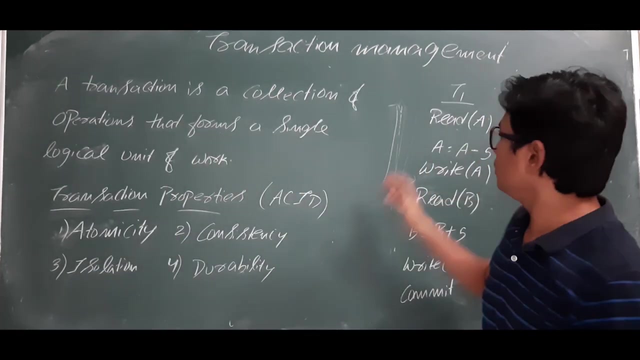 not able to further execute this. Now, what we have to do is that we have to roll back. Meaning is that you should not update this modification and you should roll back. Is it clear? So either you should execute all the operations or you should not execute any one of the operation, but you should not. 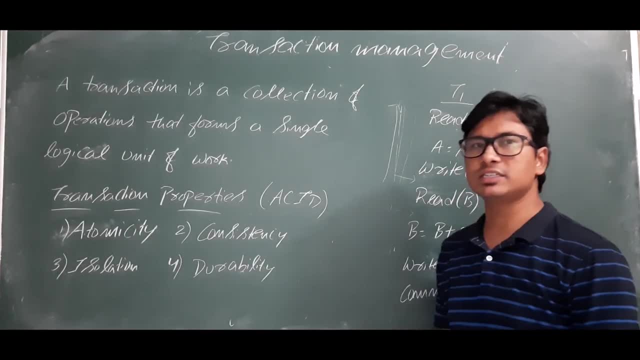 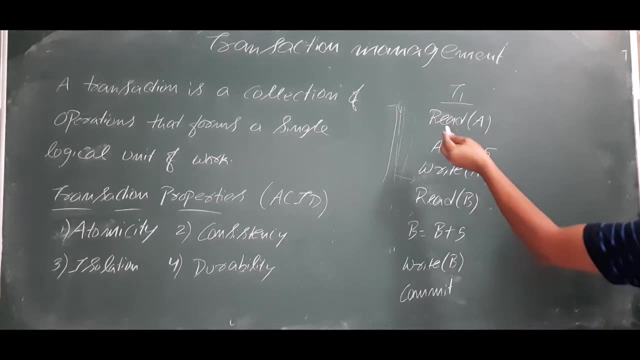 stop in between. Now come to the consistency. Consistency says that whatever the modifications you are doing, It should be consistent Suppose. to explain it proper way, I will give a small example. Let's take that A value is initially 10.. B value is 20.. If I perform A plus B Now, I will 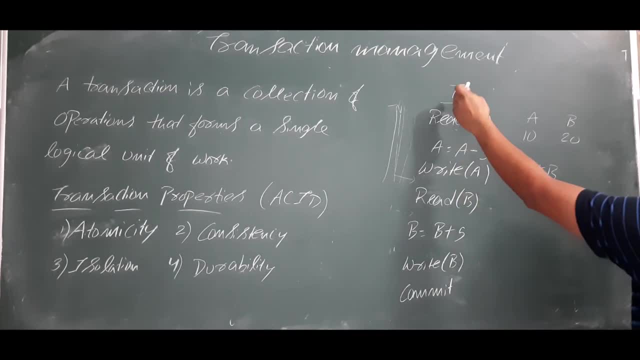 get 30. Now I started executing this transaction. Read A. I am reading the value 10. A is equal to A minus 5. Now A value will become 5.. Write A: We are saving it. Now we are saving it. 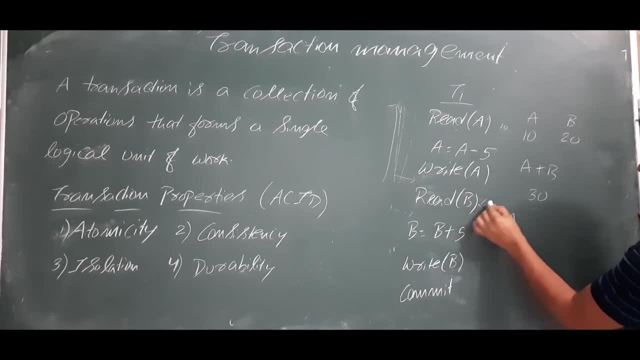 Read B, It will read the value 20.. Now B is equal to B plus 5.. Now B will be updated to 25.. Now, if I display A plus B, It is displaying 30 for me. So before executing this transaction, 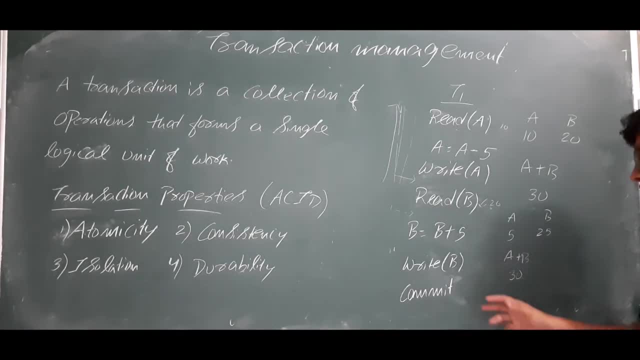 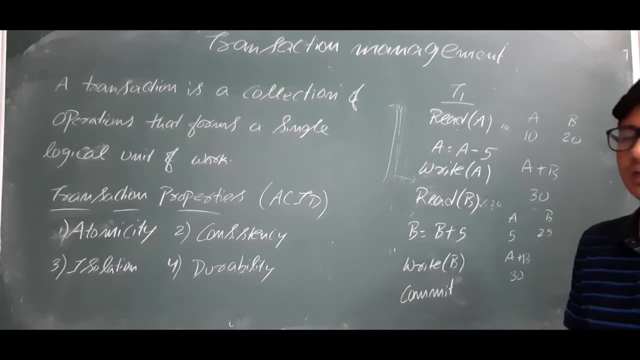 I got the A plus B is 30. After executing this transaction, also, A plus B is 30. So then I can say that this is a consistent transaction. If I am not getting the same transaction, Then I can say that this is a consistent transaction. If I am not getting the same transaction, Then 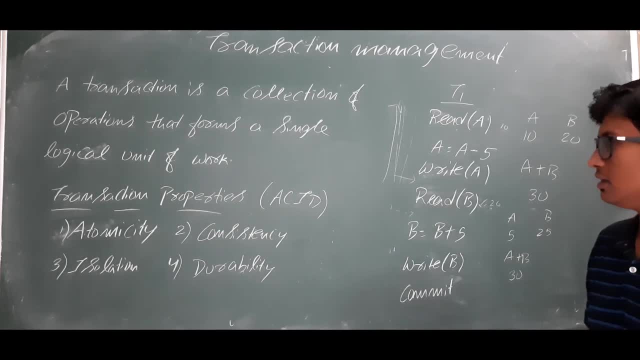 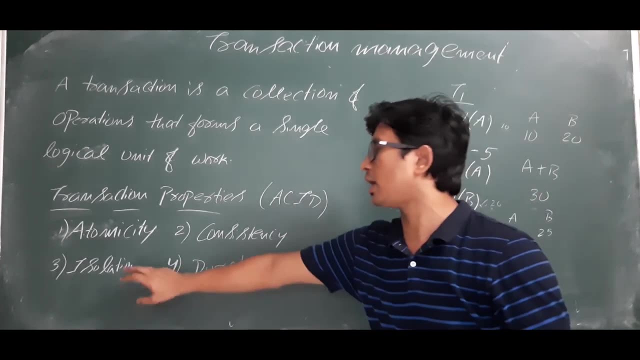 I can say that this is a consistent transaction. If I am not getting the same result, Then I can say that it is not consistent. So we have discussed about what is atomicity and what is consistency. Let me discuss about isolation. Isolation means when we are executing. 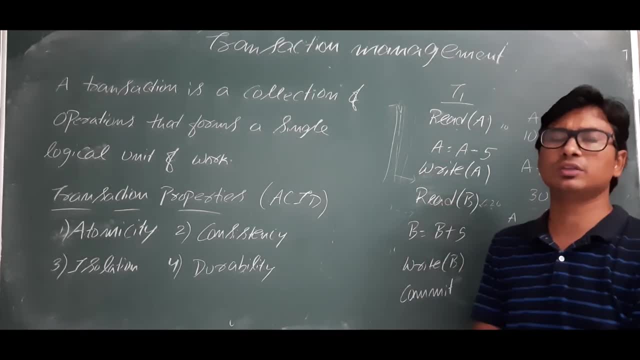 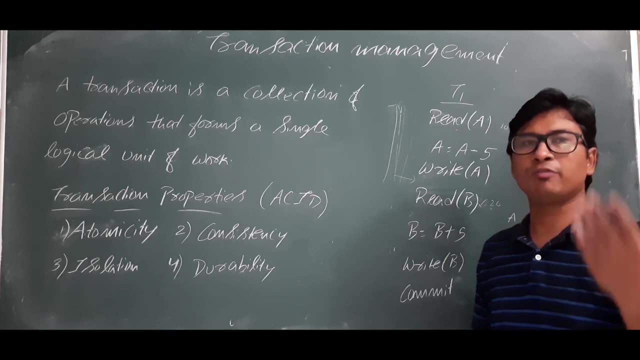 set of transactions in parallel. We will not execute the transactions in a serial way. If you execute the transactions in a serial way, we cannot increase the performance of our database. So if I want to execute all the transactions in a serial way, Then I can. 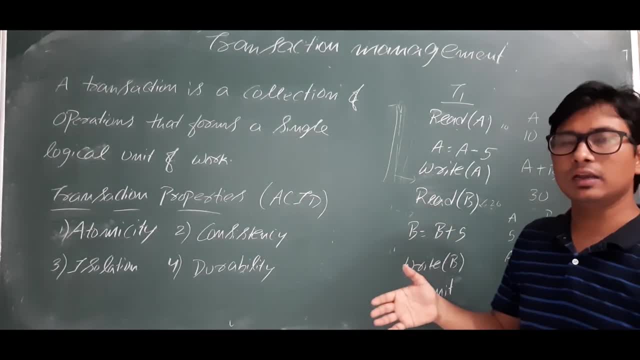 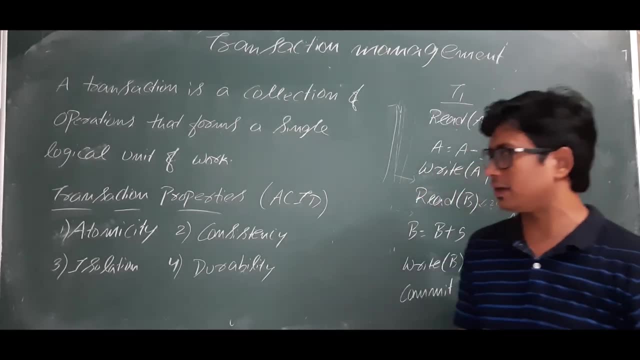 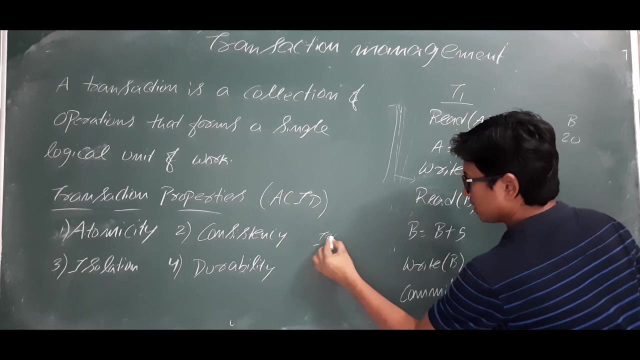 say that if I want to execute all the transactions in a parallel, but they should be executed in a isolated way. Meaning is that. let me explain with a small example for better understanding. Let's state that I am using IRCTC website But at the same time, lot of people in the 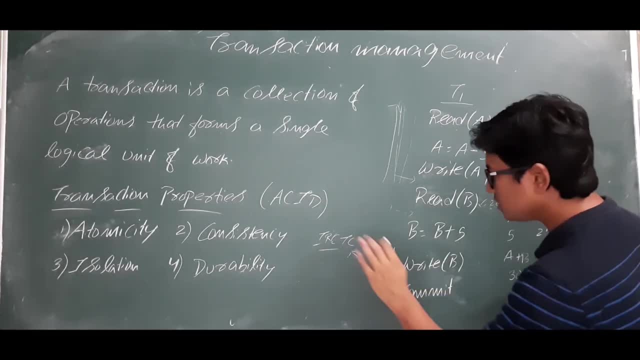 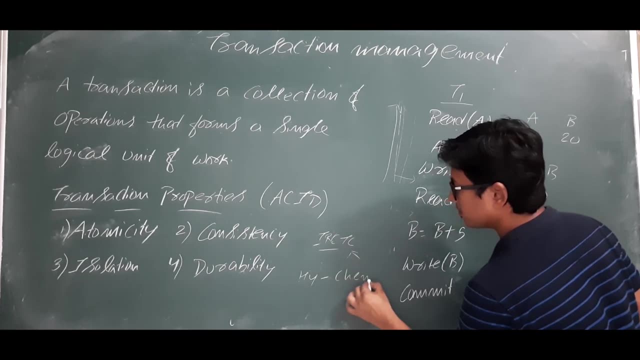 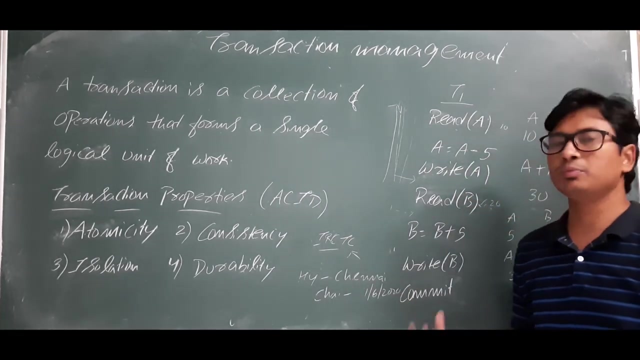 India and outside India may be using the IRCTC website. Using this IRCTC website, I want to book a ticket from Hyderabad to Chennai And I want to book a train for Charminar express on 1st June 2020.. On 1st June 2020, I want to book a ticket for Charminar express- Hyderabad. 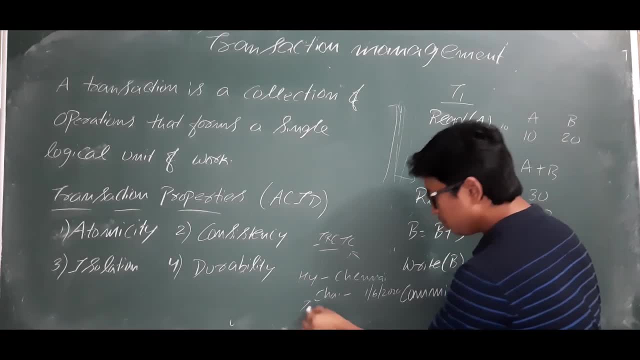 to Chennai Now, whether I alone booking at the same time, There is a chance that others are also trying to book for the same time. So I am booking for Hyderabad to Chennai. So I am booking for Hyderabad to Chennai Now, whether I alone booking at the same time. 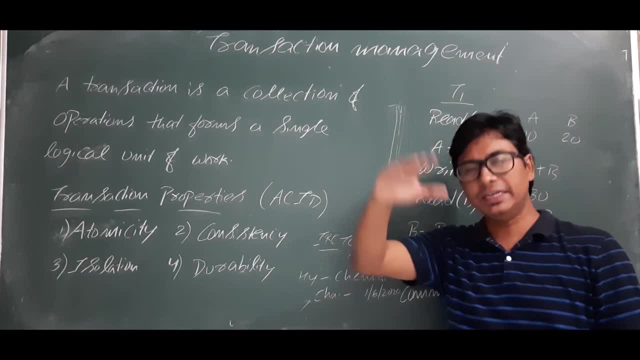 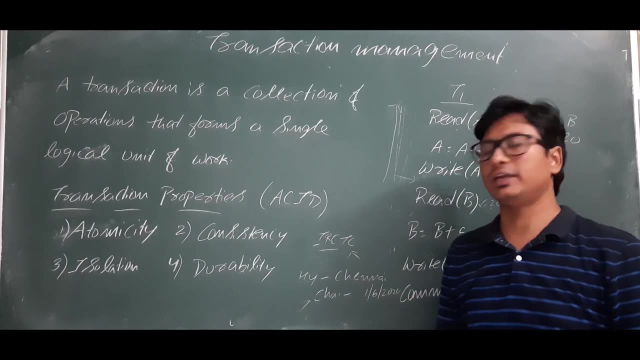 Again, I have y curseed as may be count. we could have failed, OK, But once when I am entering my details, only my details will be displayed onimly, because for me it looks like that I am only booking a train ticket for the. 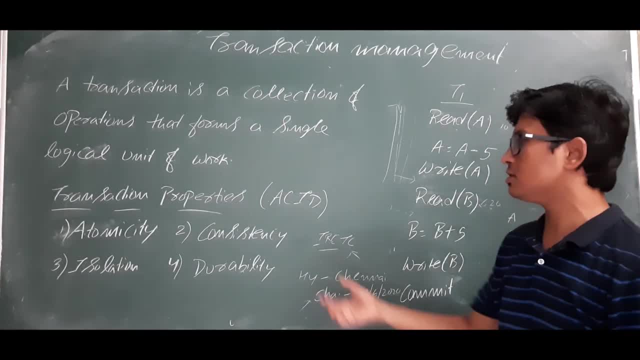 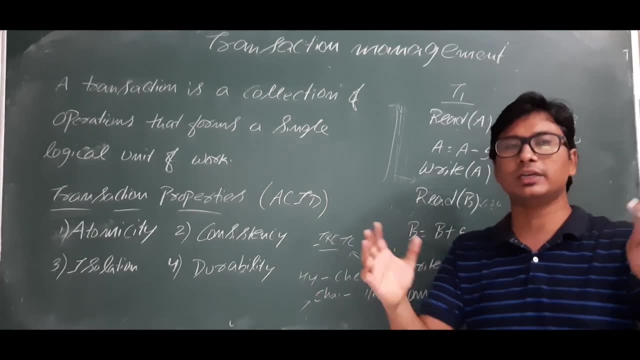 Charminar Express, but others can also book a ticket for the Charminar Express. So what I want to say? that in parallel so many transactions will be executed, but when you are executing a transaction, it should looks like that you are alone executing. So that's what we can. 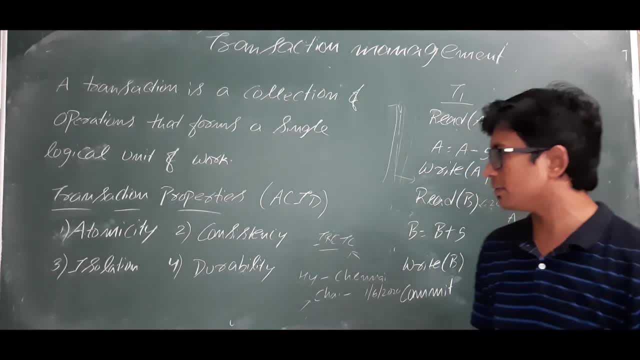 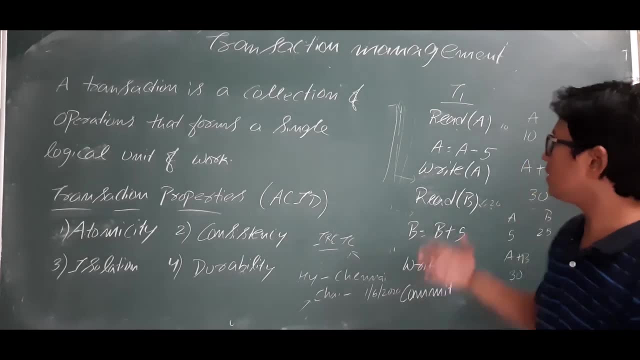 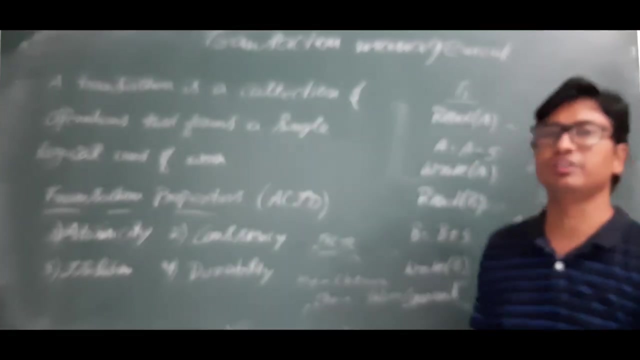 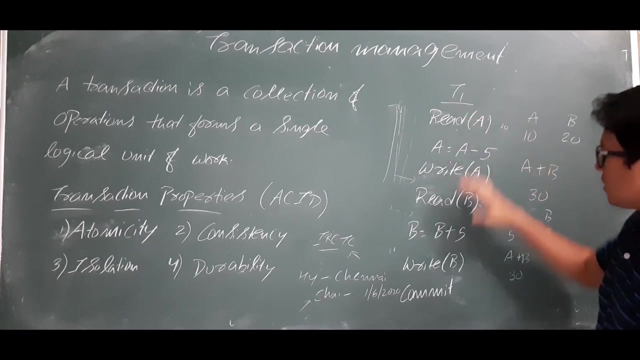 say that should be executed in a isolated way. now, what is meant by durability? durability says that what are the changes you have done on the transaction? they should be persistent. okay, even if the system fail fails also okay. let me discuss again: what is the durability? you have executed some transaction, okay. 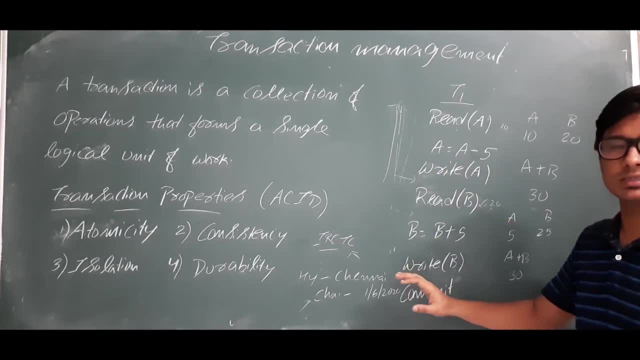 what are the changes you have done to the database? okay, you have done. the a is equal to a minus 5, so a value will become 5 and b value is 25. after executing this transaction, a is 5 and b is 25. okay, and you have performed the commit. meaning is that these values are. 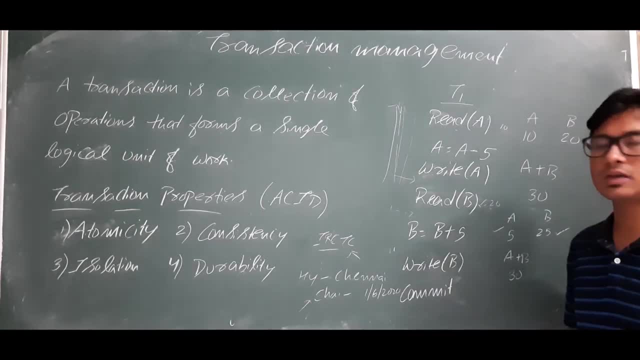 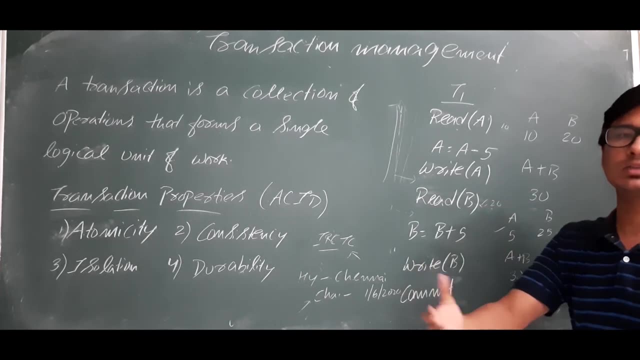 permanently stored in the database once this operation is performed. you if? what are the changes you have done to the database? you have done- the a is equal to a minus 5 and b is 25- are done in the database. they should be persistent even if the system failures in the future, so that